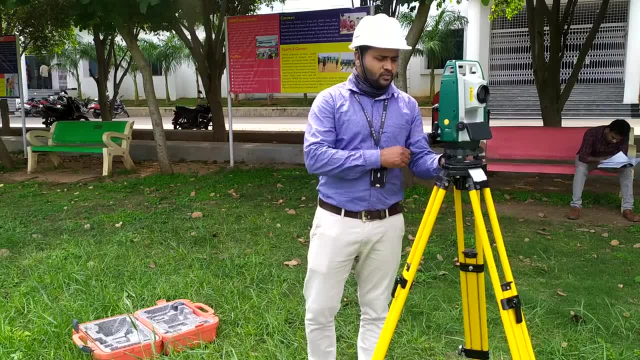 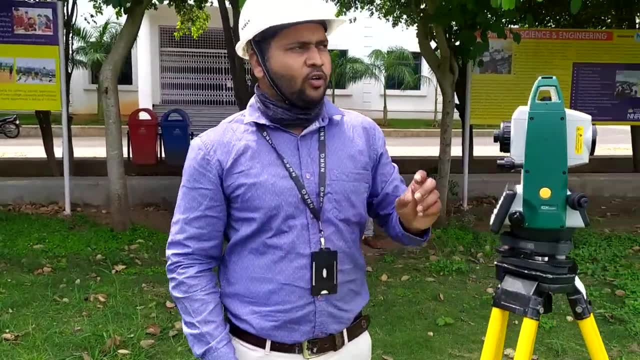 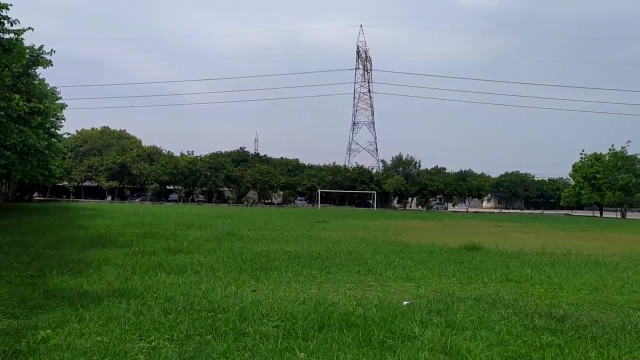 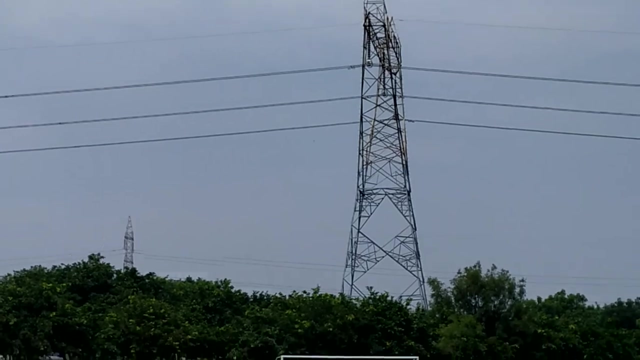 So, before going to start your experiment Now, I want to measure this height of that tower. I want to know the height of that tower because it is inaccessible to measure the height of that tower. So I am measuring that height of a tower with the help of this total station. 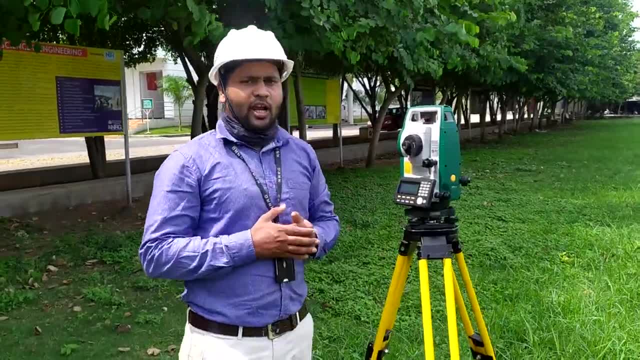 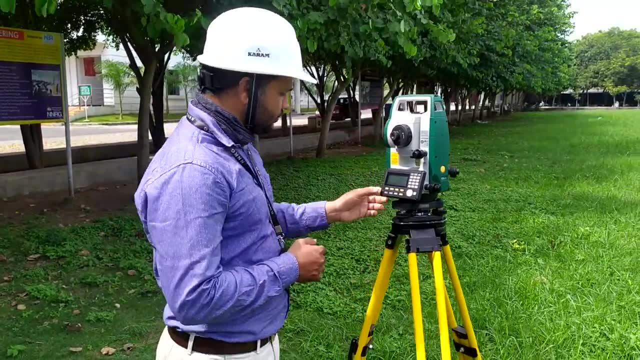 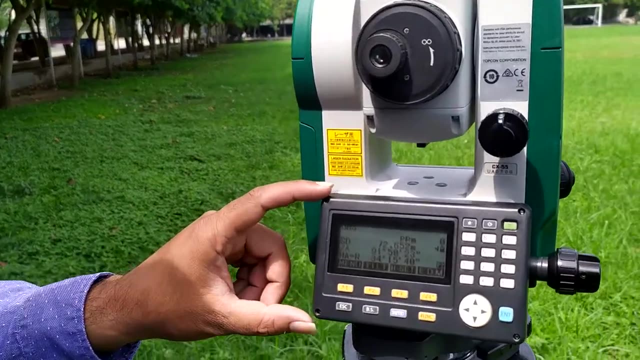 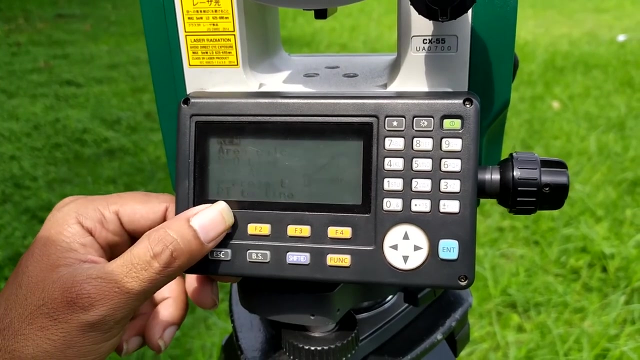 So now how to do and how to calculate that height of that tower By using this total station, We will see now. Now if you see, if you observe, on the screen of total station there will be a menu, tilt, headset and EDM. So first press F1.. 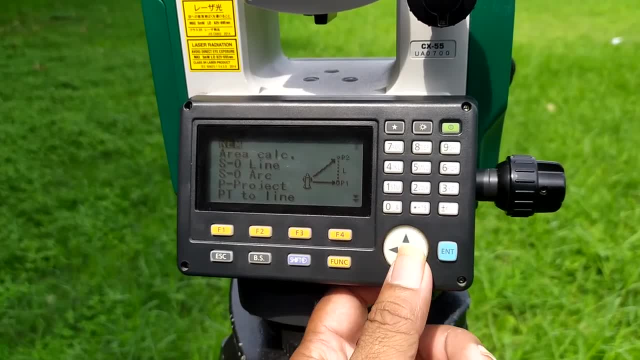 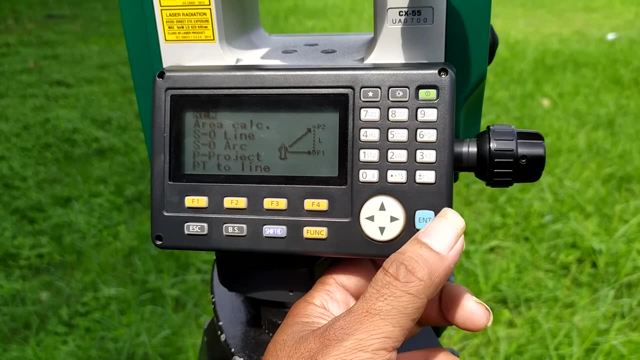 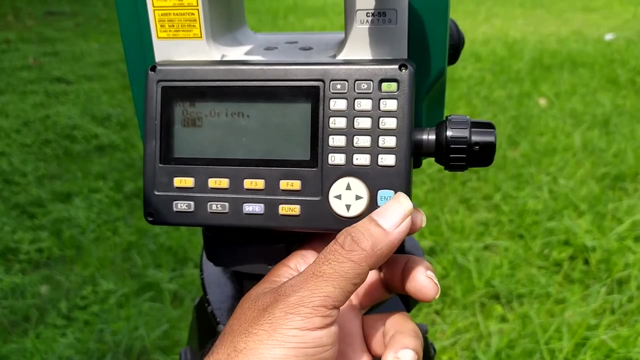 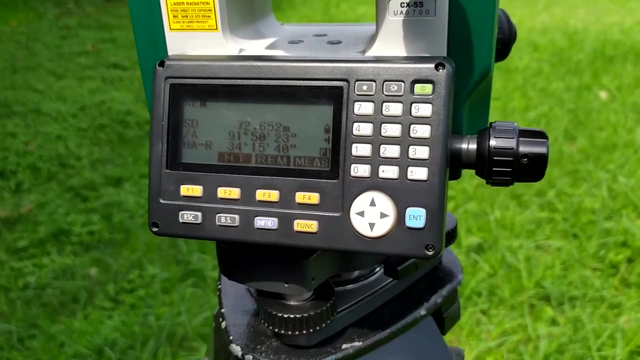 Go to REM. So if you want to calculate, area means we need to move. So today we are doing experiment REM. Enter Now again the. already the occupation orientation have been taken, So I am directly entering into REM. So here there will be options. 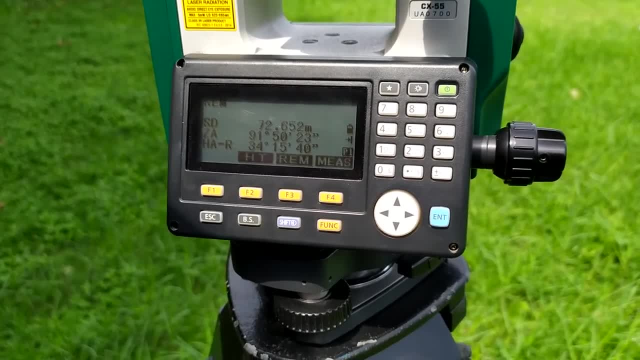 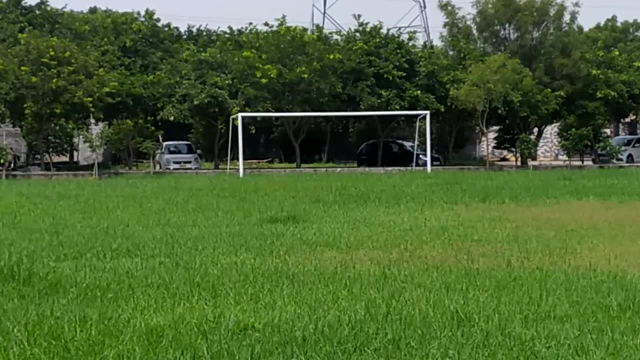 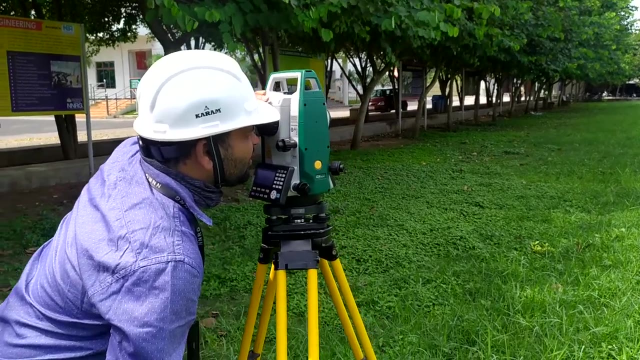 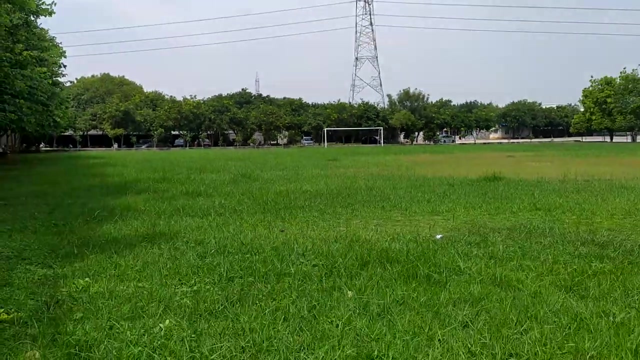 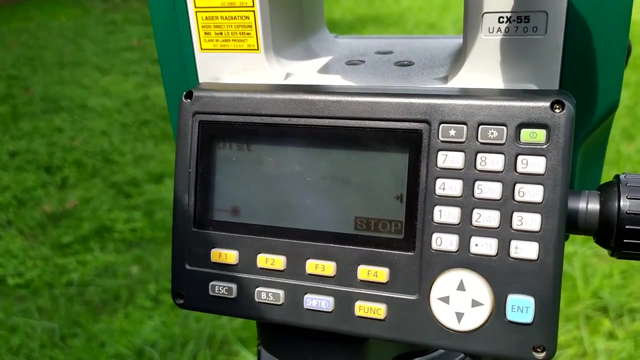 First I want to bisect the base point of that tower. So I am bisecting the base point of tower first. So I bisected the base point of a tower. I am pressing F4 button. I am pressing F4 button to measure that point. 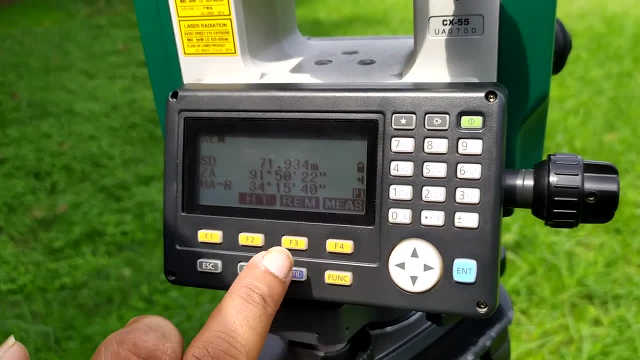 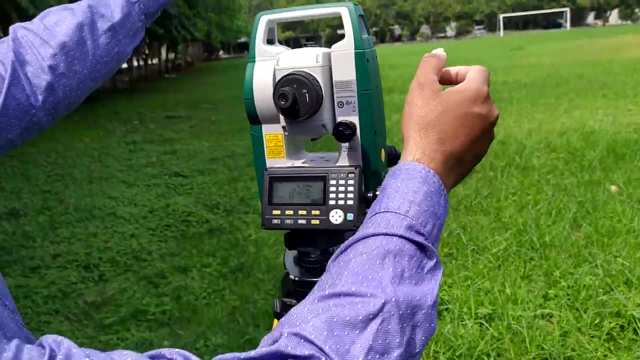 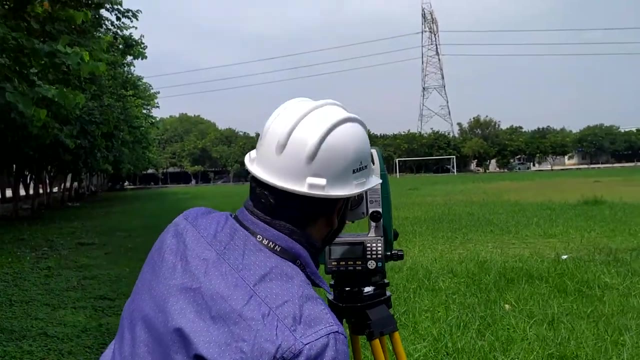 So the point have been measured. So now REM, Press REM So that we can. Now we can know the height of the tower. So I need to bisect that height of a tower with the help of this EDM, So So, 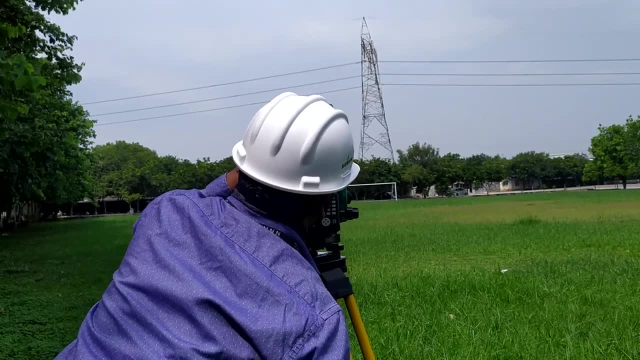 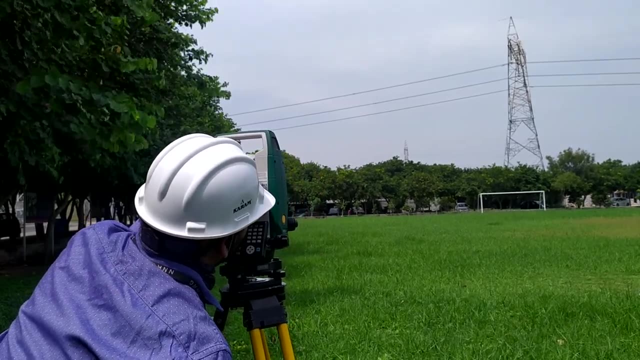 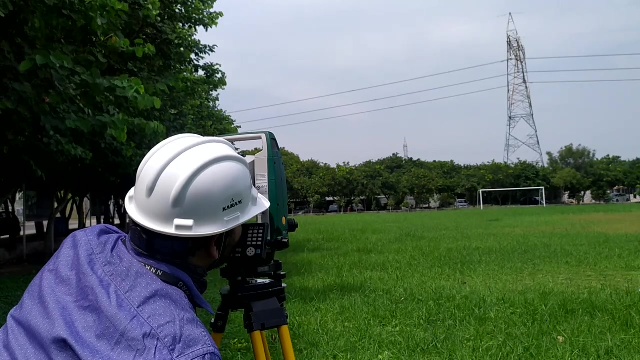